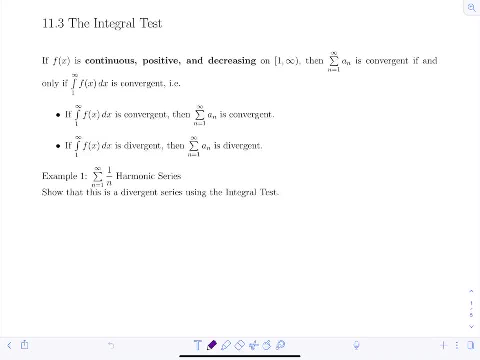 In this video we're going to be discussing the integral test, And the integral test is as follows. So if f of x is continuous positive and decreasing on the interval from 1 to infinity, then the sum from n equals 1 to infinity of a sub. n is convergent if, and only if, the integral from 1 to infinity of f of x, dx, is convergent. 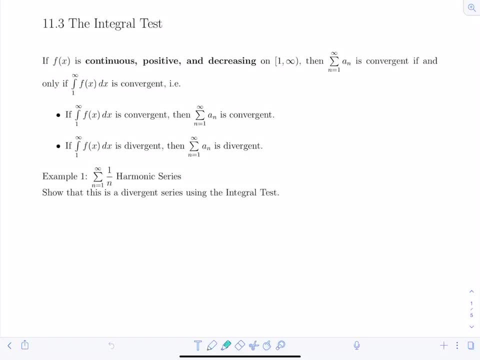 Meaning. so, since this is an if, and only if, statement, if the improper integral of f, of x, dx is convergent, then the infinite sum is also convergent, And if the integral is divergent, then the infinite sum or the infinite series is also divergent. 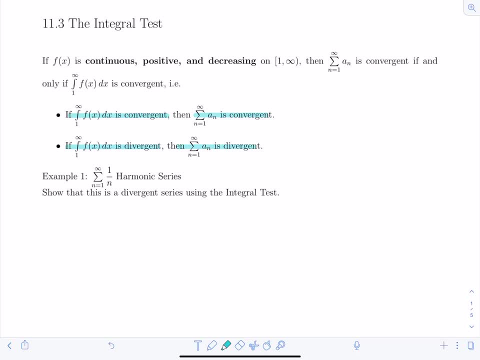 Okay, make sure, as you work on through the problems in this chapter and you learn various tests for convergence or divergence, that you memorize what conditions are necessary in order to apply them and what you need to check. And in the case with the integral test, there's three conditions. you have to check that your function is continuous, that it's positive and that it's decreasing on the interval that matches the sum of the infinite series, And then you're allowed to apply the integral test. make sure you always show that you're checking those conditions before you go ahead and apply it. So let's work through some examples so we can see how powerful this test is. 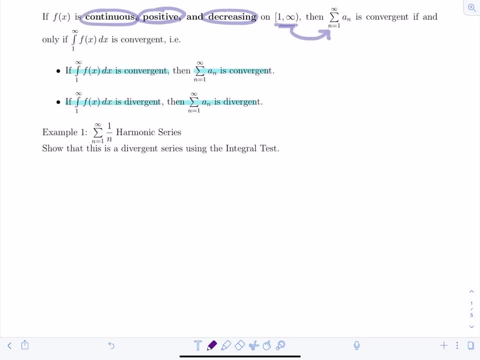 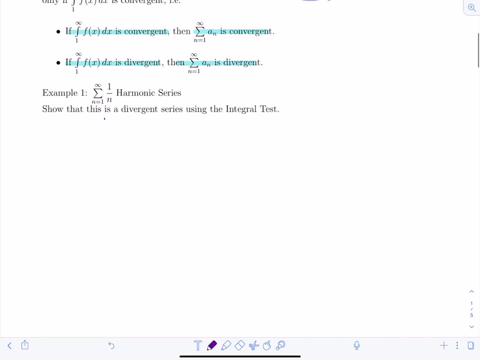 So, first example: the sum from n equals 1 to infinity of 1 over n is the harmonic series. Now, in the previous lesson we discussed the fact that this is a divergent series, And so now we're going to show this using the integral test. So what I need to do first is define a function. I'm going to let f of x equal 1 over x on the interval from 1 to infinity. So define your interval to match your limits for your index of symmetry. 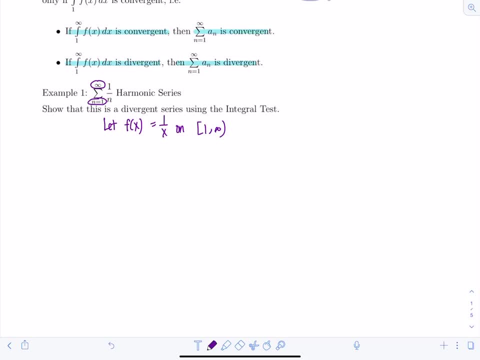 Okay. so now I'm going to check the three conditions. Is f of x continuous on the interval from 1 to infinity? Well, what's the domain of f of x? The domain is all x's, such that x doesn't equal 0. But that's fine, because I'm 1 to infinity. 0 is not included. So we're okay. Is f of x positive on that interval? Well, from 1 to infinity, I'm only subject to f of x. So I'm going to check the three conditions. Is f of x continuous on the interval from 1 to infinity? Well, what's the domain of f of x? The domain is all x's, such that x doesn't equal 0. But that's fine, because I'm 1 to infinity. 0 is not included. So we're okay. Is f of x positive on that interval? Well, from 1 to infinity, I'm only subject to f of x. So I'm going to check the three conditions. Is f of x continuous on the interval from 1 to infinity? Well, what's the? 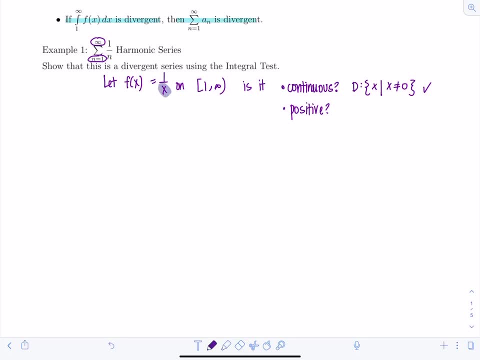 constituting in positive values for x. So yes, that's going to be satisfied. And then is f of x decreasing on that interval? Well, let's check. Let's evaluate f prime of x. Well, f of x is x to the negative first power, So f prime is going to be negative. 1 over x squared- x squared is always positive, So negative. 1 over x squared is going to be negative, So it's decreasing. since the derivative is negative, Since all three conditions are satisfied, then 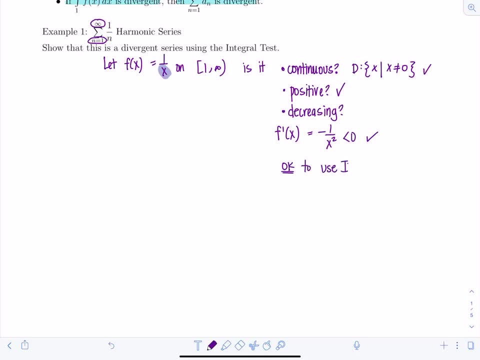 this means it's okay to use the integral test. All right, so for a complete solution, you need to show testing, all three of these conditions and a complete justification. Now let's set up our integral. So we have the integral from 1 to infinity of 1 over x dx. Now this is an improper. 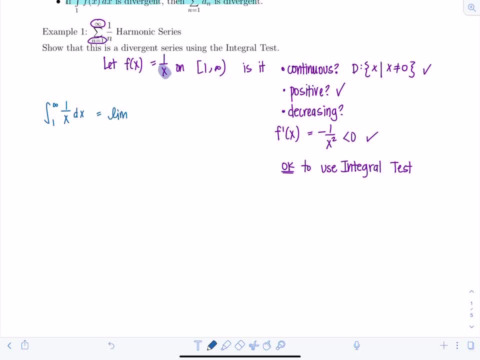 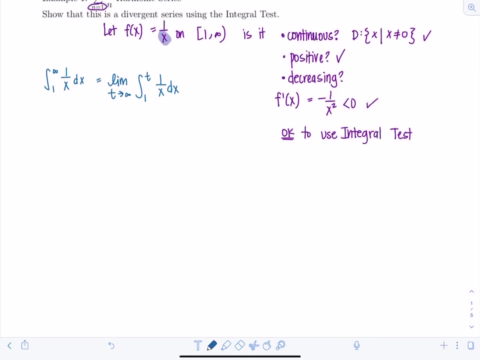 integral. So the very first thing I need to do is rewrite this as the limit as t approaches infinity of the integral from 1 to t, of 1 over x, dx, All right, antiderivative of 1 over x, that's one we're very familiar with. It's natural log of absolute value of x. So we have the limit. 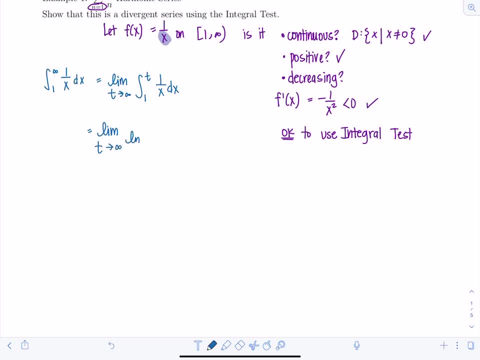 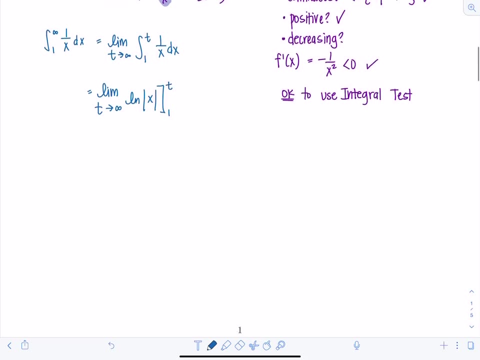 as t approaches infinity of the natural log of the absolute value of x, And I'm going to evaluate this from 1 to t. All right, so we have the limit as t approaches infinity of natural log. I'm going to substitute in t for x, So natural log of t minus natural log of 1.. 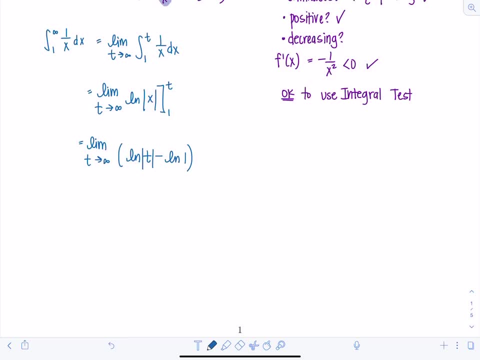 Let's keep the absolute value there, All right. so as t approaches positive infinity, then natural log of t- think of the graph of natural log- it's going to approach positive infinity And natural log of 1, that just equals 0. So this limit as t approaches infinity of 1 to 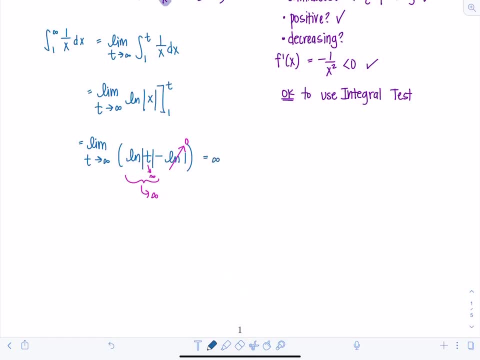 t approaches infinity is equal to positive infinity And, if you'll recall from studying improper integrals previously, we said that this improper integral diverges. Well, what does that mean for us? This means that the series or the sum n equals 1 to infinity. of 1 over n also diverges. 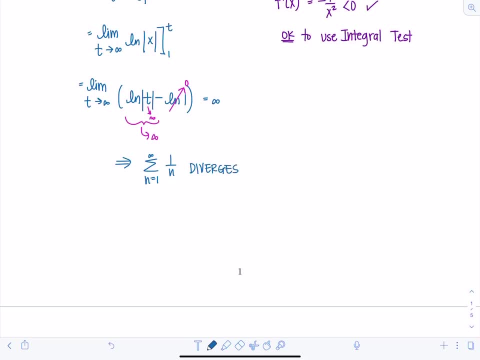 And you must state what test you just used, So by the, the integral test. All right, and as we mentioned before when we were looking at the harmonic series, even though the terms are decreasing 1 over n, that's 1,, 1 half, 1, third those terms. 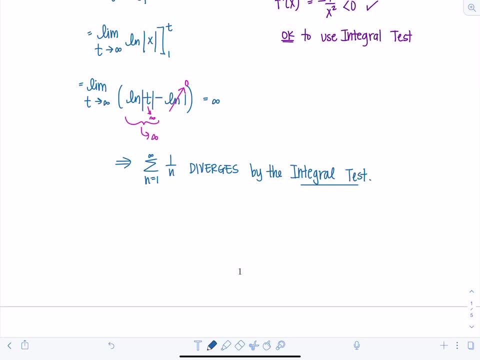 are decreasing, They're not decreasing fast enough so that their sum converges, And that's the issue with the harmonic series. Okay, now let's investigate from another series very similar. So we're going to compare f of x equals 1 over x and g of x equals 1 over x, And we're going to compare. 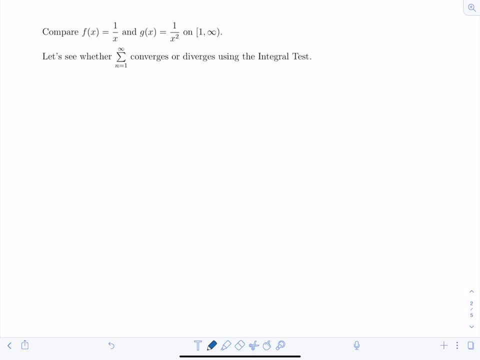 f of x equals 1 over x, squared on the interval from 1 to infinity, And then we're going to see whether the infinite sum converges or diverges for g of x. So to begin our investigation or comparison, let's graph both of these just on 1 to infinity. So I'm only going to draw. 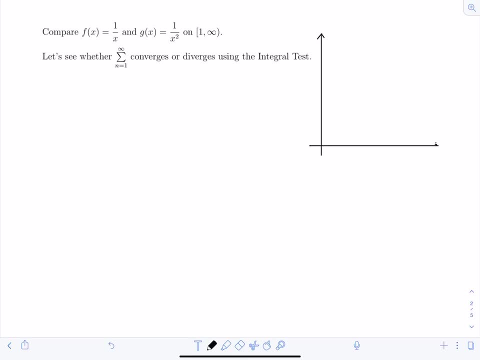 values in the first quadrant. Okay, here's x, here's y, And maybe we'll just plot the first four. Okay, so f of x is 1 over x. So 1 over 1 is 1, 2 is going to be a half, 3 is a third, maybe here. 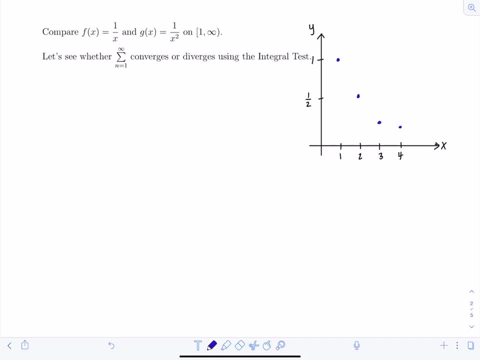 and 4 is a fourth. Okay, so this is f of x. Now g of x is 1 over x squared, So they'll have the same initial value here. But at 2, g of x is going to equal 1 fourth. At 3, g of x is going to equal 1 ninth. At 4, 1 sixteenth. So we can see. 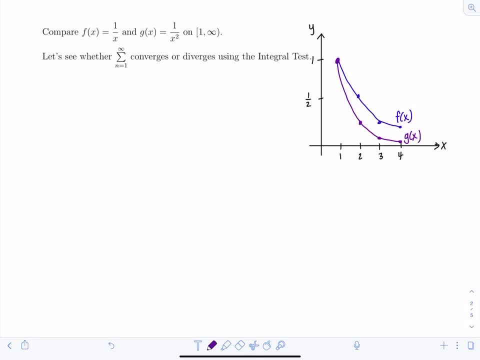 g of x is decreasing a lot faster than f of x, So do you have any suspicions or guesses as to what's going to happen with this? Okay, so we have g of x equals 1 over x, squared on the interval from 1 to infinity. Now is it? 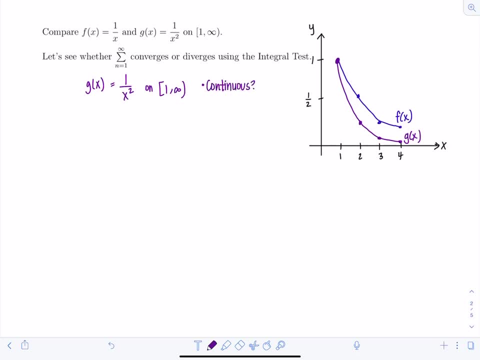 continuous. We have to check our three conditions. Well, yes, it has the same domain, all x's, such that x doesn't equal 0. So it's going to be continuous. on 1 to infinity: Is it positive? Well, yes, 1 over x squared is always going to be positive, especially on the interval from 1 to infinity. Okay, so we have g of x equals 1 over x, squared on the interval from 1 to infinity, And we have g of x equals 1 over x, squared on the interval from 1 to infinity. And lastly, I need to check- 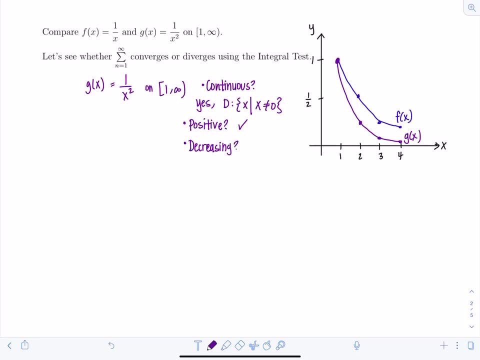 is it decreasing? Well, let's compute the derivative again. So g prime of x is going to equal. so 1 over x squared, that's x to the negative second. So this is going to be negative 2 over x cubed. Remember you're only substituting in values from 1 to infinity for x, So that's. 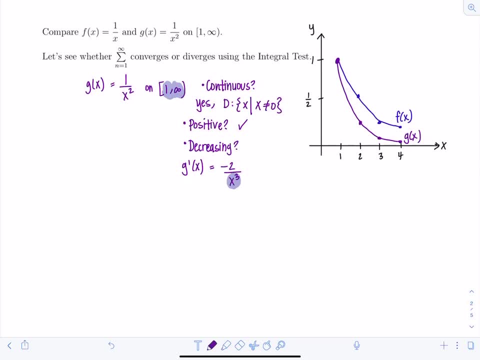 always going to be positive, And so negative 2 over a positive number. this is going to be negative for all x's that are elements of the interval from 1 to infinity. So we have g of x from 1 to infinity. So, yes, it's decreasing. So all three conditions checked out, this tells me. 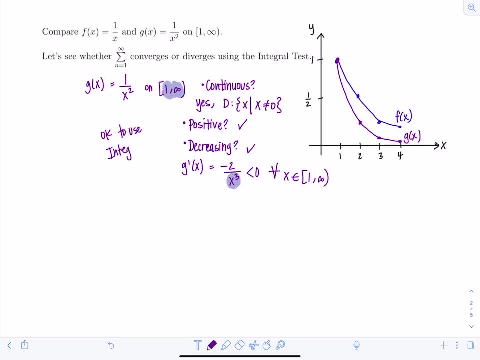 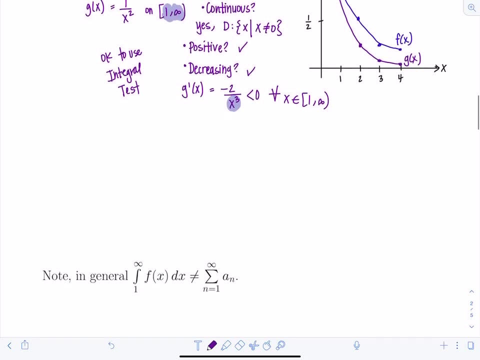 it's okay to use the integral test. All right, so let's go ahead and do it. Let's set up our integral, So we have the integral from 1 to infinity of 1 over x squared dx, Right away. very first thing, rewrite this as the limit as t approaches. infinity of the integral from 1. 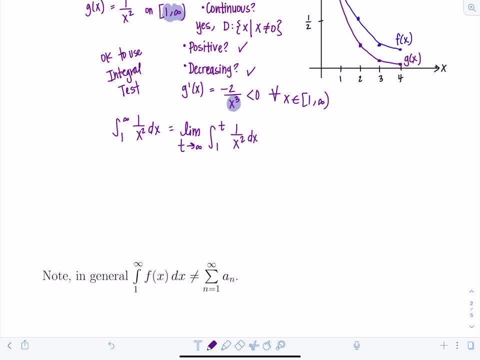 to t of 1 over x squared dx, which equals the limit, as t approaches infinity, of negative 1 over x, right x to the negative. second antiderivative is going to be negative x to the negative first, and then I'm going to evaluate that from 1 to t. So this is going to be the limit. 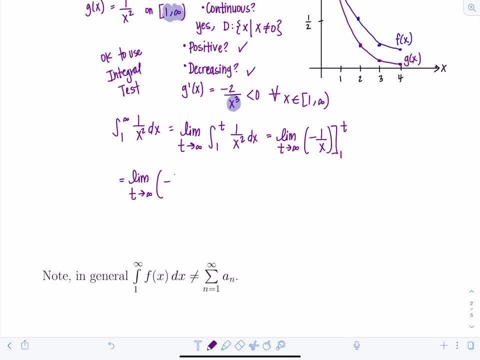 as t approaches infinity, of negative 1 over t plus 1 over x squared dx, Right, minus negative 1.. And then, as t approaches infinity, well, negative 1 over t is going to approach 0. And so this equals 1.. Well, what does this tell me? Well, remember from previous: 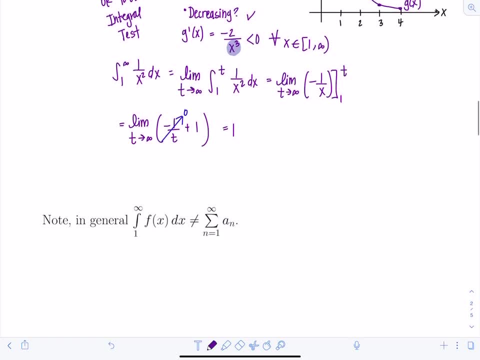 chapters. this means our improper integral converges And by the integral test we know that our infinite series, so the sum n equals 1 to infinity of 1 over m squared, also converges by the integral test. All right now note in general, whatever value you get for the improper integral. 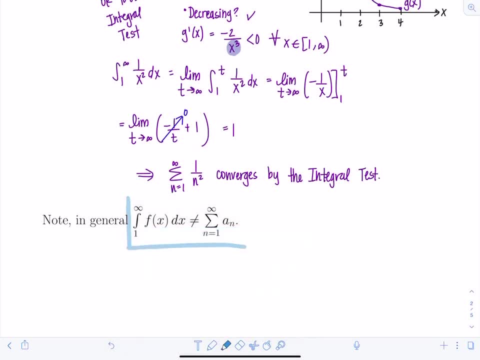 it's not equal to the infinite sum. Okay. so for example here, when we evaluated the improper integral for 1 over x squared dx, the value of that came out to be 1.. b, k x 1. but that's actually not what the sum of 1 over n squared is, from 1 to infinity. 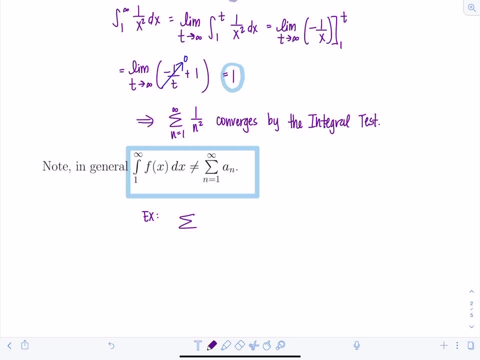 In fact, the sum, from n equals 1 to infinity, of 1 over n squared is equal to pi squared over 6.. And if you ever take complex analysis, you'll see how you can find that sum. So notice, it's not equal to 1.. All the integral test tells us is whether it converges or diverges. 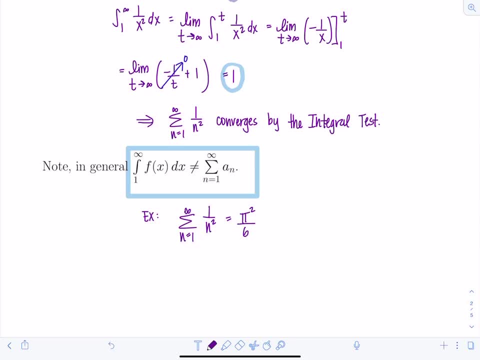 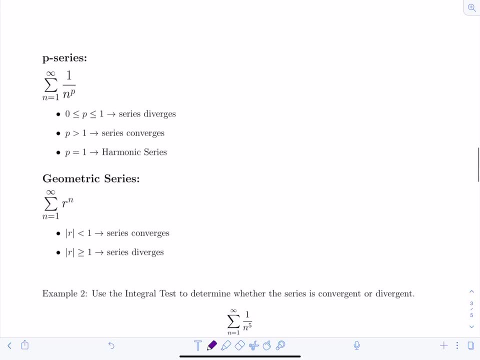 but not necessarily what it will sum to Okay. so now let's recap a little bit. Noticing here, the harmonic series diverged, but 1 over x squared or 1 over n squared converged, And that's because we can call them p-series, much like we did when we were looking at improper integrals. 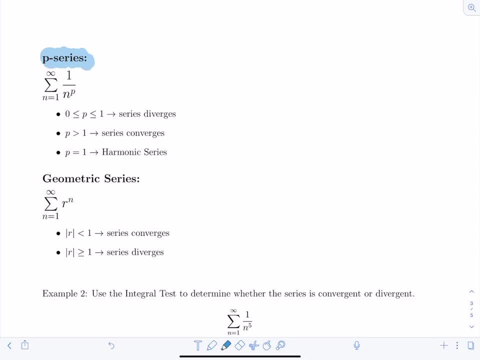 So if you have the sum n equals 1 to infinity of 1 over n to the p right, So if this exponent here, p, is between 0 and 1 inclusive, then the series diverges. So that includes the harmonic series when p equals 1.. 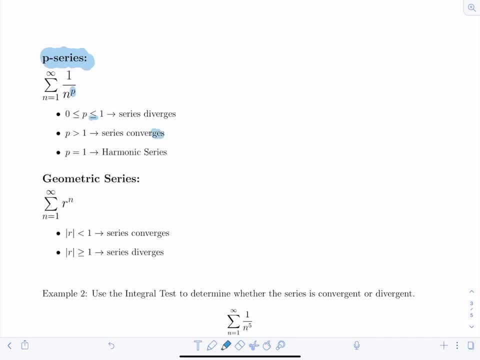 If p is greater than 1, then the series converges. That was like 1 over n squared that we just looked at here. What that means is when p is greater than 1, that's causing the denominator to grow faster, so the series is shrinking fast enough in order to converge as an infinite sum. 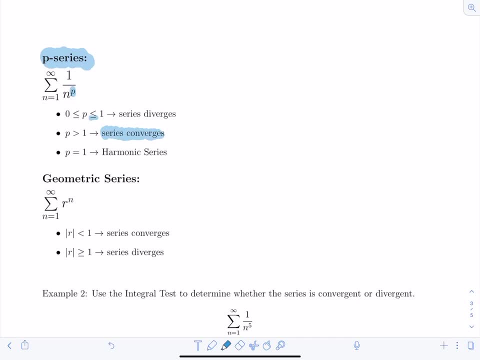 And if p equals 1, it's the harmonic series. So from here on out, most of the time, as long as you just identify that a sum is a p-series, you don't have to go through any testing in order to justify whether it converges or diverges. 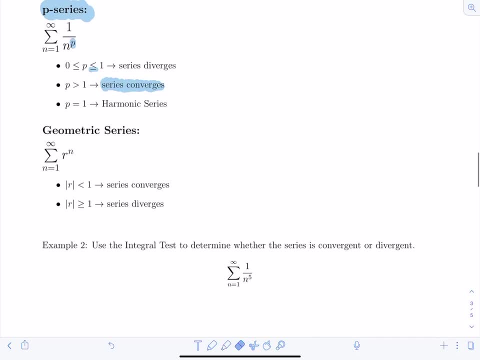 And then, if you'll recall before, don't get this confused with geometric series- where you have r raised to the n And if absolute value of r is less than 1 over n squared, then the series converges, And if the absolute value of r is greater than or equal to 1,. 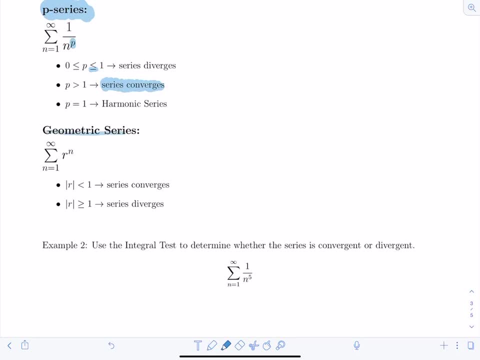 then the series diverges. And remember, geometric series, if they converge, are very, very special because we are able to in fact compute their sum, their infinite sum. All right, Remember s equals a1 over 1 minus r, only if it converges. 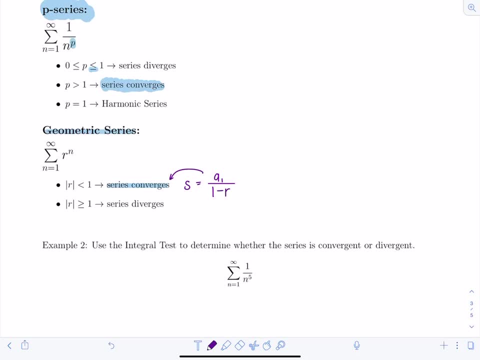 All right, Let's look at one more example of a p-series. Here the directions say: use the integral test to determine whether the series is convergent or divergent. Okay, Can you already tell what's going to happen? I mean, this is a p-series. 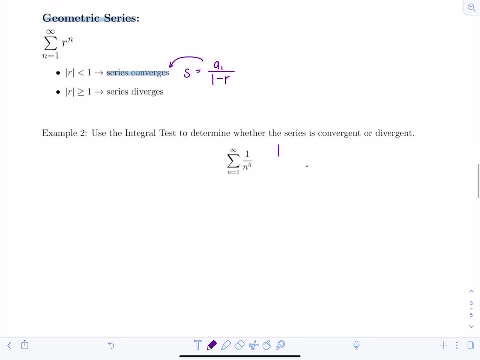 And p is equal to 5, right? So this is a p-series. p equals 5,, which is greater than 1, which means the series converges. However, we're going to do a p-series. However, we're going to do a p-series. 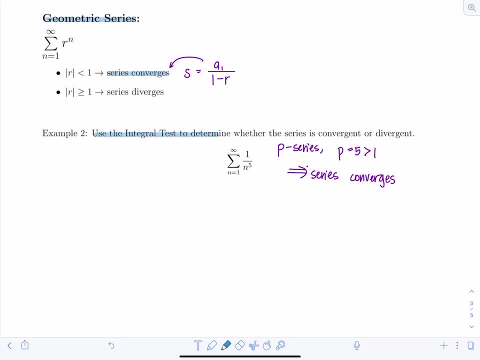 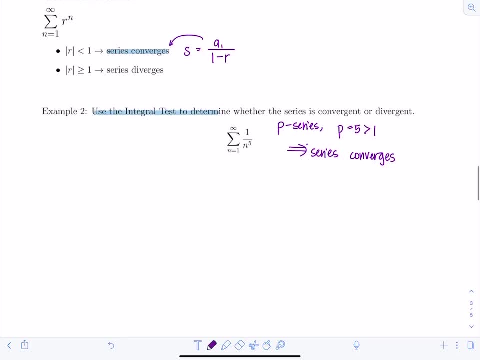 But it's nice to know what we should expect the outcome to be. So we're going to let f of x equal 1 over x to the 5th on the interval from 1 to infinity, And let's check our three conditions. 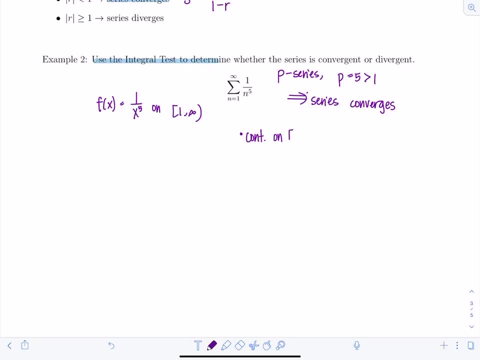 So, first, is it continuous on 1 to infinity? Well, yes, The domain is all real values of x, such that x doesn't equal 0. So we're good on the interval from 1 to infinity. So we're good on the interval from 1 to infinity. 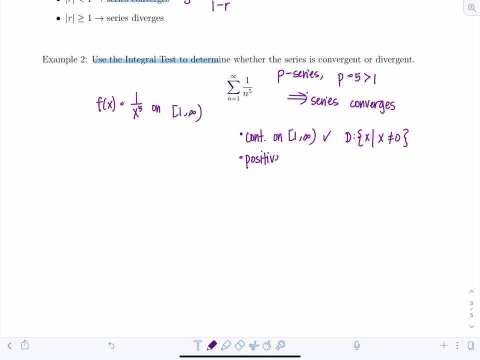 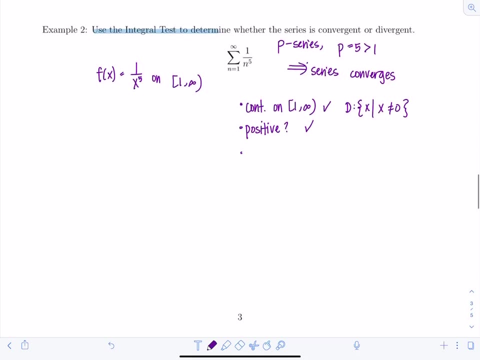 So we're good on the interval from 1 to infinity. Is it positive on the interval from 1 to infinity? Yes, it is. I'm only substituting in positive values for x. And then is the function decreasing. Well, let's check its derivative. 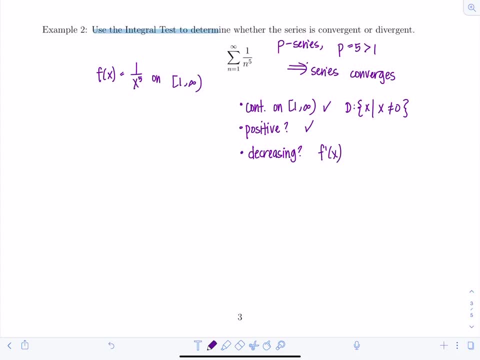 So f prime of x- Remember f of x is x to the negative 5th, So f prime is going to be negative 5 over x to the 6th And this is definitely less than 0.. Denominator is always positive. 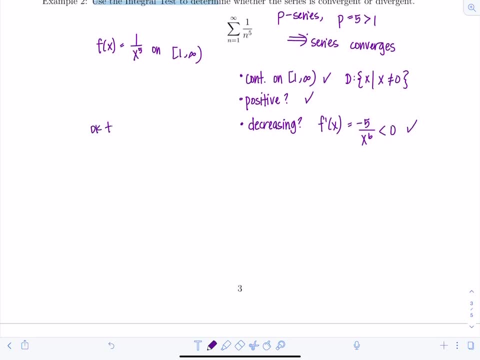 Numerator is always negative. So that means it's okay to use the integral test And let's go ahead and set up our improper integral. So we have the integral from 1 to infinity, of 1 over x to the 5th dx. 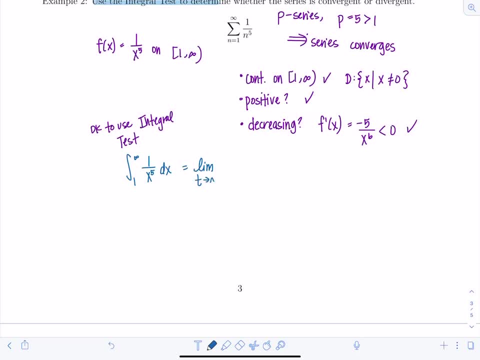 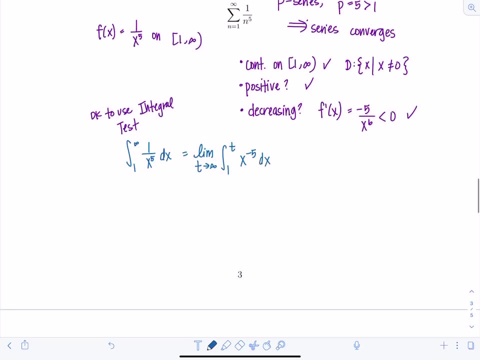 I'm going to rewrite this as the limit, as t approaches infinity, of the integral from 1 to t, x to the negative 5th, dx, And then let's go ahead and anti-differentiate. So this is going to be the limit. 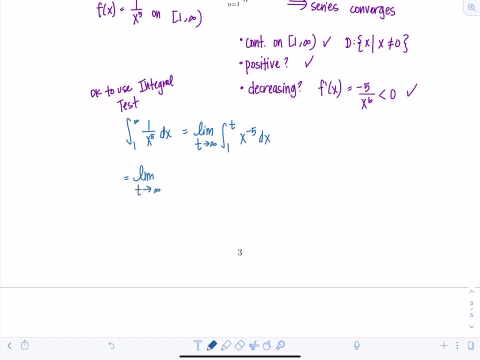 This is the limit as t approaches infinity. I'm going to have x to the negative 4th, so I'm going to have a negative 1, 4, t, x to the negative 4, evaluated from 1 to t, And this equals the limit as t approaches infinity. 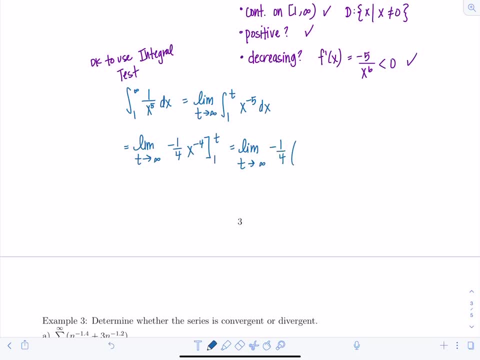 I'll leave the negative 1 4th factored out and then I'm going to substitute, in my limits of integration. so x to the negative 4, substituting t for x, I'm going to have 1 over t to the 4th minus 1.. 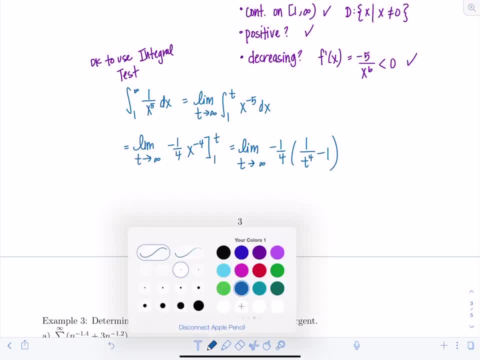 minus 1.. And then now I can take this limit. So as t approaches infinity, 1 over t to the fourth is going to go to 0.. All I'm left with now is negative 1, fourth times negative 1.. And this is. 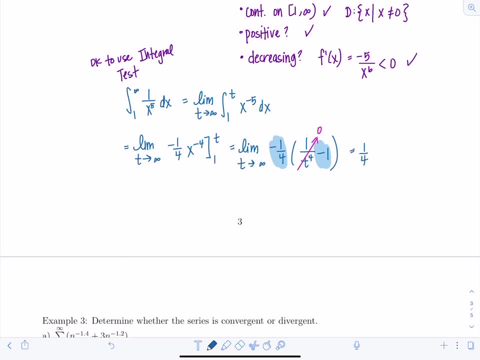 going to leave me with a positive 1. fourth, So since this is a finite number, right, that means the improper integral converges. So the sum n equals 1 to infinity of 1 over n to the fifth also converges by the integral test. Make sure anytime you're testing for convergence, or 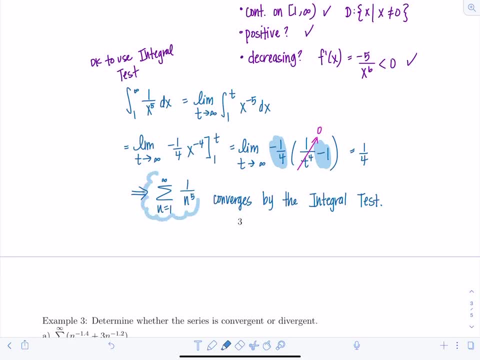 divergence of a series, you rewrite the original series in your statement, You clearly write out if it converges or diverges, and then you also include the test. Okay, this is something you need to get into the habit of doing throughout the chapter. 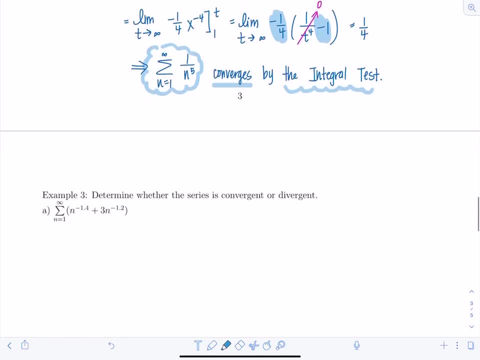 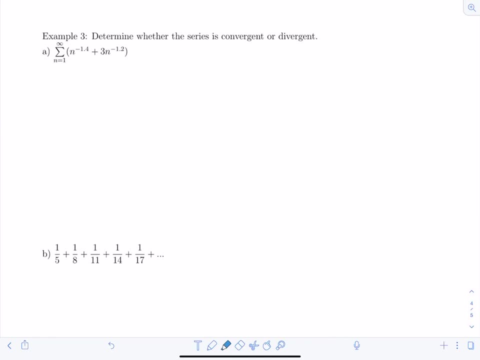 Okay, now a few other examples. Notice here: now the directions just say to determine whether the series is convergent or divergent. So they're not instructing us what test or method we need to use. It's up to us. So notice, here I have the sum. n equals 1 to infinity, of n to the negative. 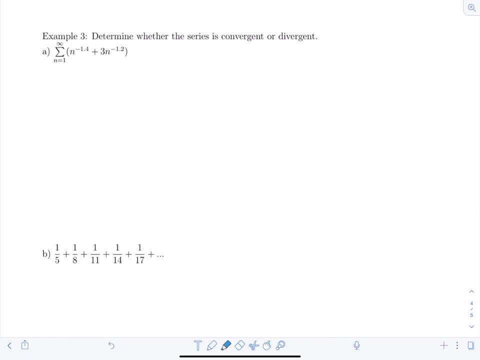 1.4 plus 3n to the negative 1.2.. Now what I'm going to do is separately consider each of these terms as individual infinite series And determine whether or not they converge or diverge before I can make a statement about the. 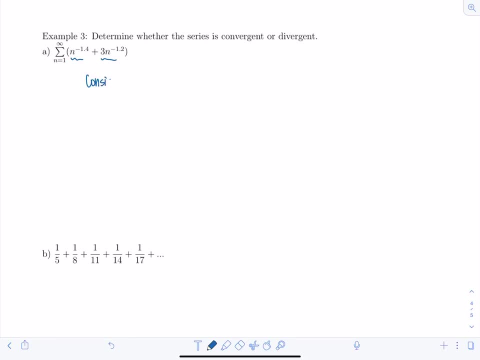 original. Okay, so first I'm going to consider the sum n equals 1 to infinity of n. to the negative 1.4.. And notice, that's a p-series. I can rewrite this as: the sum n equals 1 to infinity of 1 over. 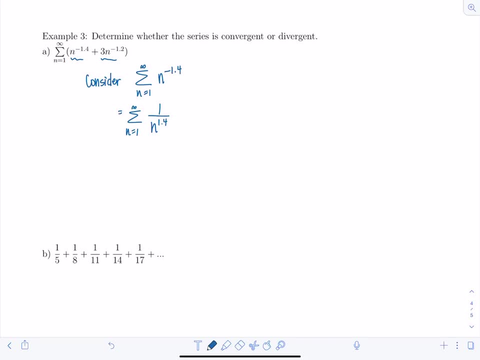 n to the 1.4.. So here's how you would use the fact that it's a p-series. You're going to first state that, Hey, this is a p-series. What is p? Well, p is 1.4. And guess what? That's bigger than 1.. And what? 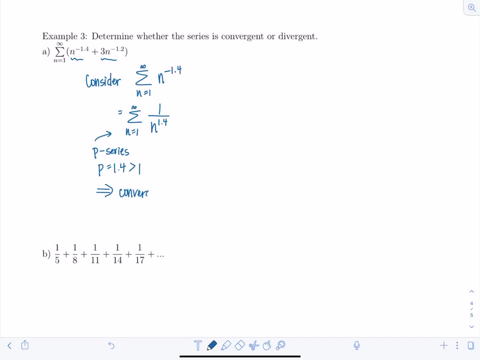 does that tell me? This means that the series converges. Okay, so make sure, if you're not going to go through the whole integral test, which you really shouldn't. okay, then you clearly state: this is a p-series, identify what p is, compare it to 1, and then state your conclusion. 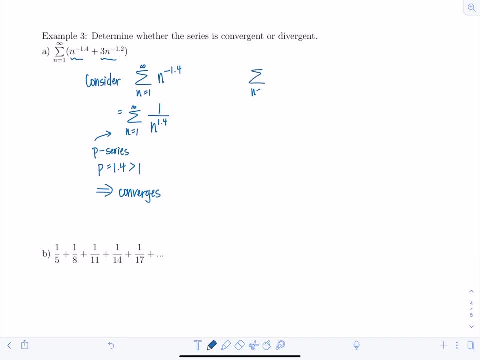 Okay, now I'm going to consider the next part. the sum n equals 1 to infinity of n to the negative 1.4.. I can take the 3 outside, so 3 times the sum n equals 1 to infinity of 1 over n to the 1.2.. Notice: 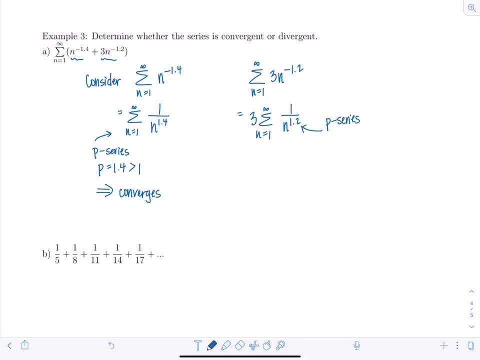 this is also a p-series. What is p? p is 1.2, and that is greater than 1.. So this series also converges, And if you have an infinite series that converges, it's a p-series, So you're going to. 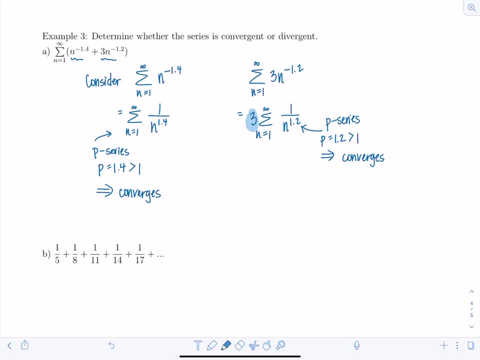 multiply by a constant, it's still going to converge. If you have a series and it diverges and you multiply by a constant, it's still going to diverge. So you can always pull out a constant and it will not affect the convergence or divergence of a series. Okay, so what can I say? 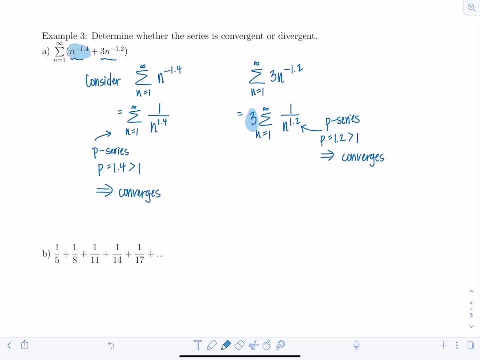 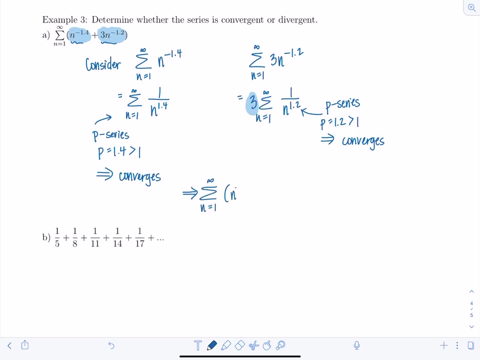 now, since I know this part of our sum converges as well as this part. Well, now I can put them together. right, We have one of our infinite series properties, a theorem from earlier that said this means that the sum n equals 1 to infinity, of n to the negative 1.4.. Rewrite the original exactly how you saw it, Okay. 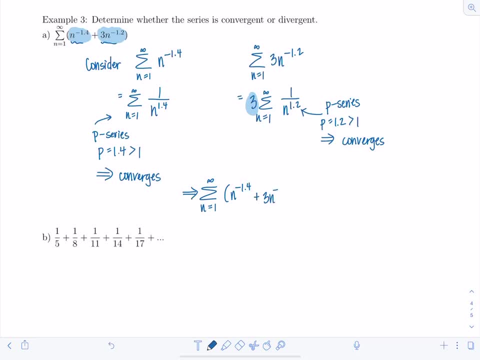 don't change a thing. Plus 3n to the negative, 1.2 also converges, All right, nice. Now don't be lazy, don't just say, oh converges, or draw an arrow. You must rewrite the original exactly as you saw. 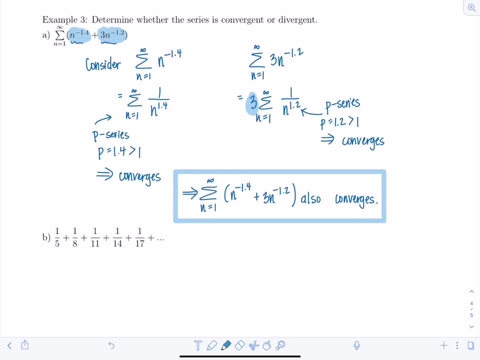 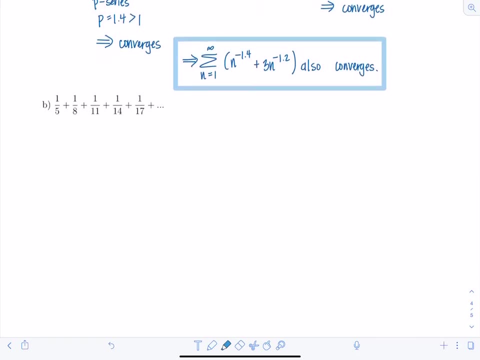 it Beautiful. Okay, let's look at this, This next series here. notice they didn't write it for me in summation notation. They've just listed out the first few terms, So let's investigate what's going on. So we have 1- 5th. 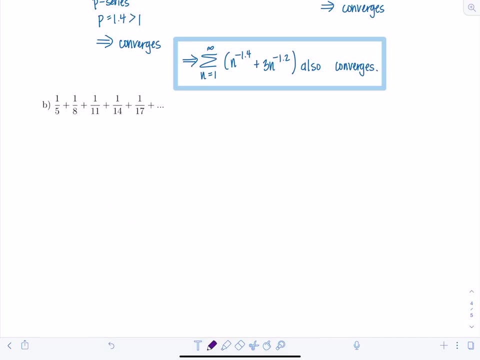 plus 1 8th plus 1 11th. I noticed the denominators each time are going up by three. Okay, so that means this is not geometric right. I'm not multiplying by a common ratio And I don't. 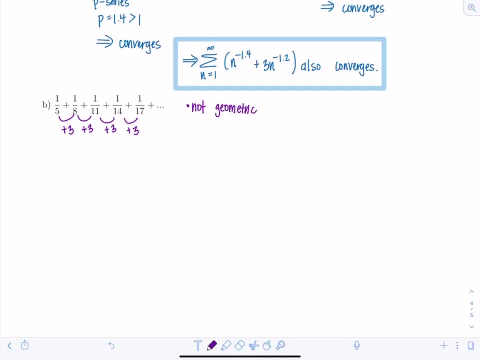 I don't see any signs alternating right with positives and negatives. So this is not a telescoping sum, like we saw in the last section, And it's not a p-series. P-series is, if you see, n squared, n cubed, some power of n in the denominator. 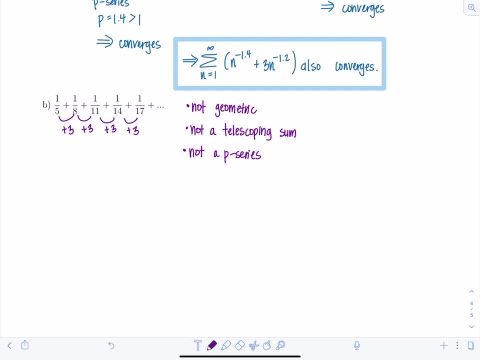 Can you write this out in summation notation? Maybe that'll help us get a feel for what's going on. Denominator is always increasing by three. You could just treat the denominator as an arithmetic sequence and then just put one over whatever expression you get. So notice, I can write this: 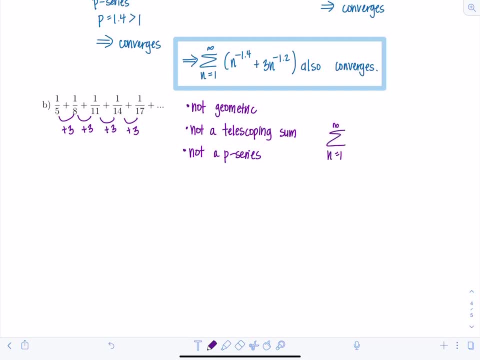 as the sum n equals 1 to infinity. Since the denominator is going up by three every single time, you're going to have 3n, And then if you want the very first term to have a five in the denominator, then 3 times n, 3 times 1, would just give me 3.. So I better add 2 and then put 1 over. 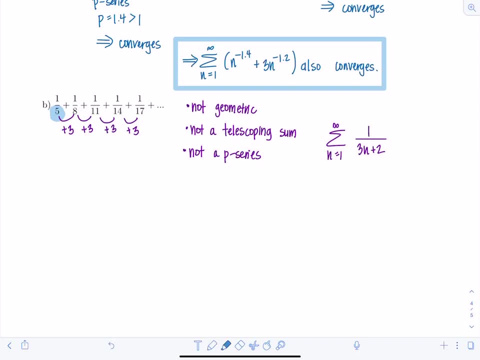 that And that checks out right. You can confirm If I substitute n equals 2, that would give me the second term, etc. Ooh, that's not what I wanted. Okay, So all of the methods that we're thinking- geometric, telescoping, p-series- don't apply. 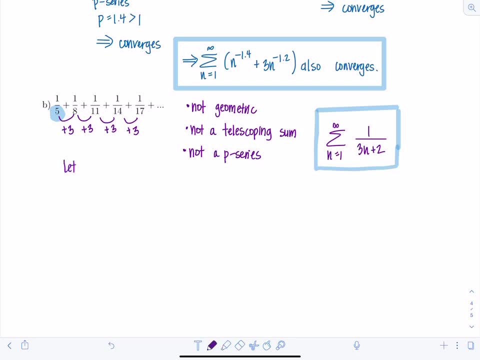 Well, let's try the test for divergence I mentioned in the previous video. you always want to check this first, at least mentally, even if you don't write it out. Let's try the test for divergence, or divergence test, meaning I'm going to take the limit. 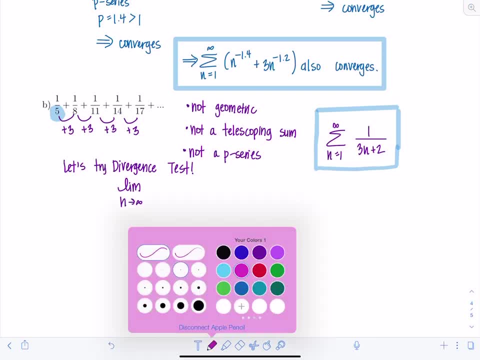 as n approaches infinity of a sub n, of just the terms 1 over 3n plus 2.. What is that limit? It's zero. So what does that tell me? Nothing. This is inconclusive, Remember. the test for divergence only gives you information. 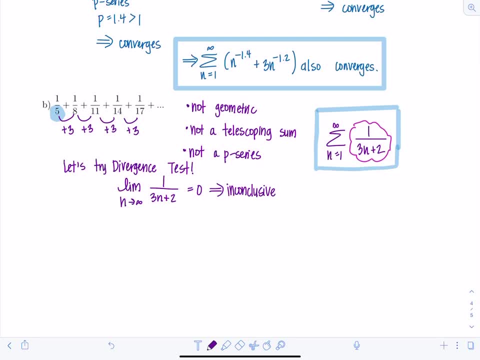 if the terms do not go to zero, Then you can say: oh for sure, my infinite series diverges. If the terms aren't going to zero, there is no way I could add them all up and have the sum converge, right. 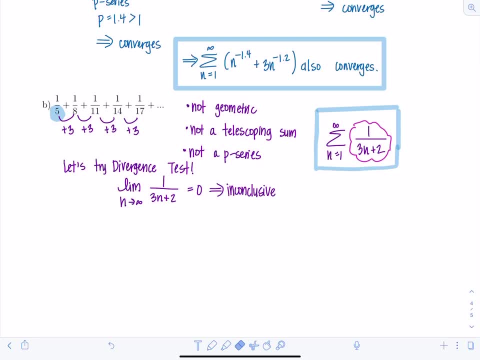 The terms at least have to go to zero. But if they go to zero, that doesn't give us any info. That's a necessary but not sufficient condition for convergence. All right, I'm all out of options, So let's try the integral test, Why not? 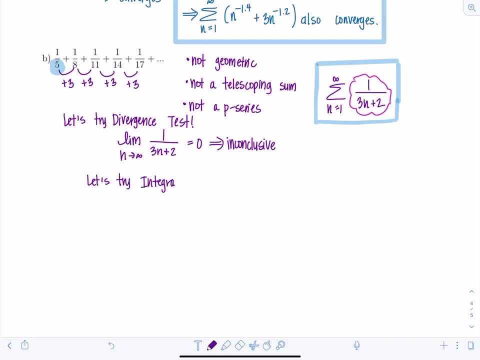 That's the only thing we have left at this point, So let's try the integral test. All right, I have to check the conditions. So we're going to let f of x equal 1 over 3x plus 2. And I want to confirm: OK, is it continuous on the interval from 1 to infinity? 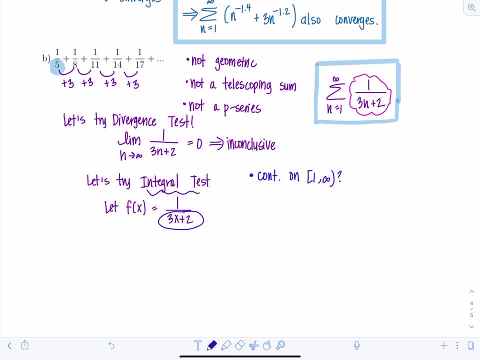 Well, what's the domain for this function? here I could see it's going to be undefined at negative two thirds. So the domain is all x's, such that x doesn't equal negative two thirds. But we're fine, It's going to be 1 to infinity, right? That's not going to be a problem for us. 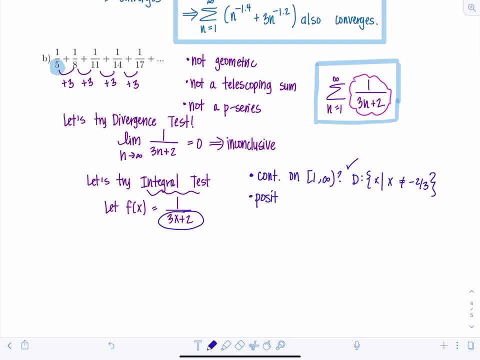 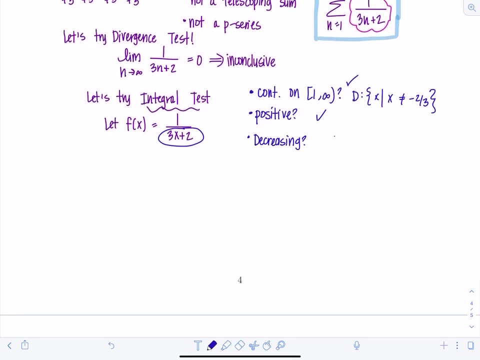 So we're good. Is it positive on that interval? Well, yes, If I'm only substituting in 1 to infinity for x, we're good to go, And then is it decreasing. So again, I want to compute f prime of x in order to check. 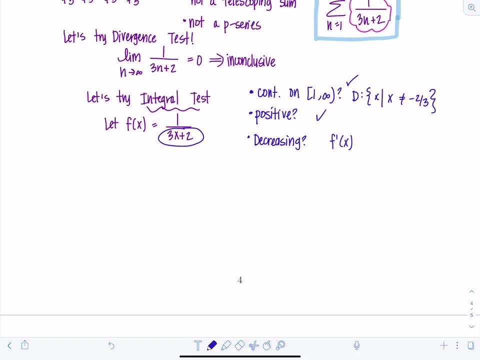 Now, f of x is 3x plus 2 to the negative first power, right. So the derivative is going to be negative And I'm going to have 3x plus 2 squared, And then, by the chain rule, I need a 3 in the numerator. 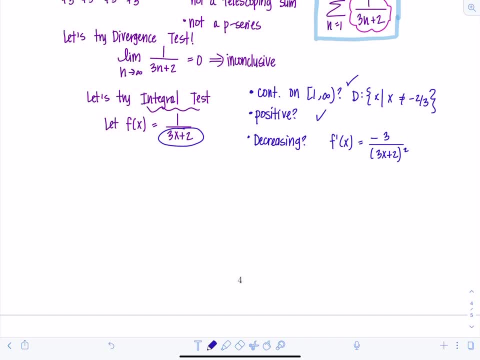 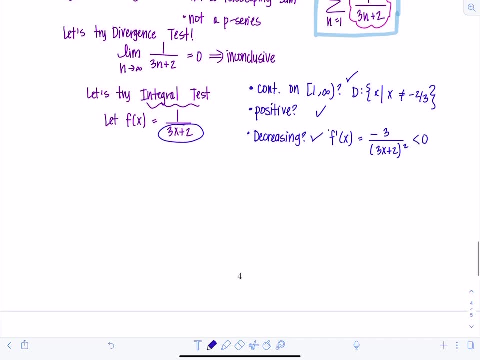 Well, the denominator is squared, so that's always positive, And then the numerator is going to be negative, So this is for sure less than 0.. So, yes, my function is decreasing, So that means we can use the integral test. 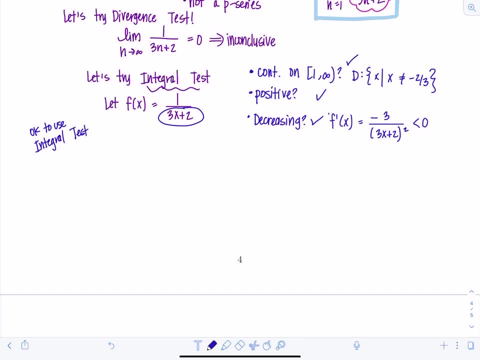 Fabulous, OK. So let's write out our improper integral. We have the integral from 1 to infinity of 1 over 3x plus 2 dx, and this equals the limit as t approaches infinity of the integral from 1 to t of 1 over 3x plus 2 dx. OK, 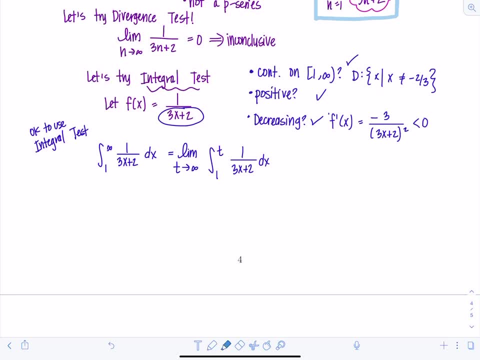 Now come on. At this point you don't need to do a full u-sub. If I were to let this denominator equal u, then du would have a 3 dx attached to it. So I would have to divide right by 3 or multiply by a 1- 3rd. 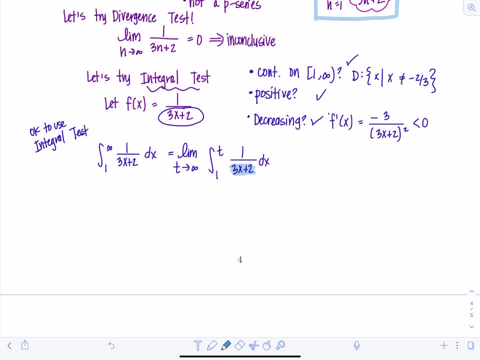 So just add the 1- 3rd here and anti-differentiate appropriately, So we're going to have the limit, as t approaches infinity, of 1- 3rd times the natural log of the absolute value of 3x plus 2.. 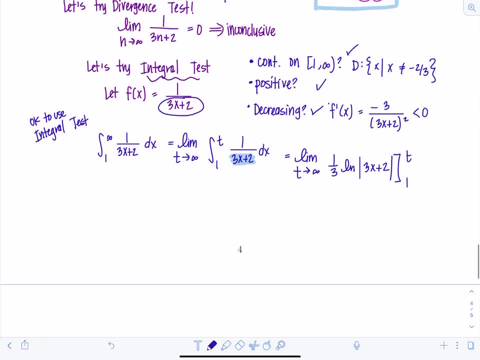 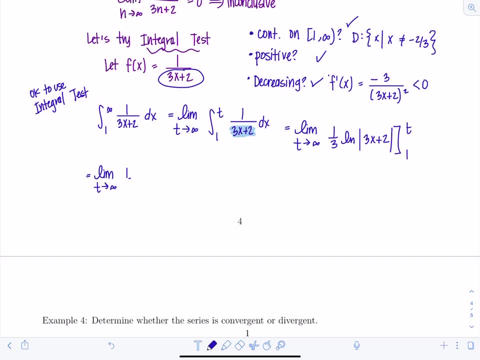 evaluated from 1 to t. All right, And then now I'm going to substitute in my limits of integration. So this is the limit, as t approaches infinity, of 1. 3rd, We have natural log of the absolute value of 3t plus 2, minus natural log. 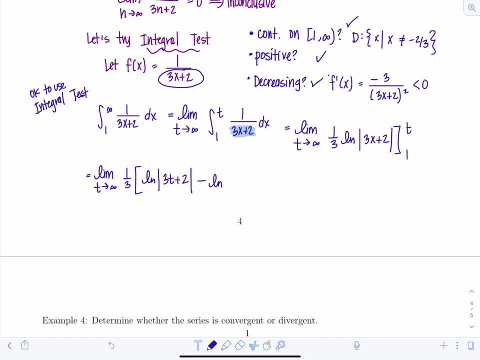 If I substitute in 1 for x, that's going to be 3 plus 2, so ln of 5.. All right, Now let's see As t approaches infinity: 3t plus 2, that's going to go to infinity. 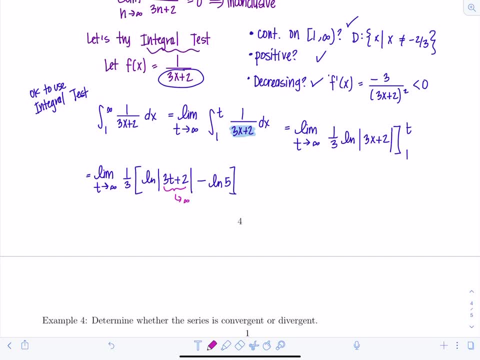 So natural log of infinity. think of the graph. This is going to all approach infinity. ln of 5 is just a constant. So infinity minus a constant. this whole thing is just blowing up. So this limit is equal to infinity. So what does that tell me? 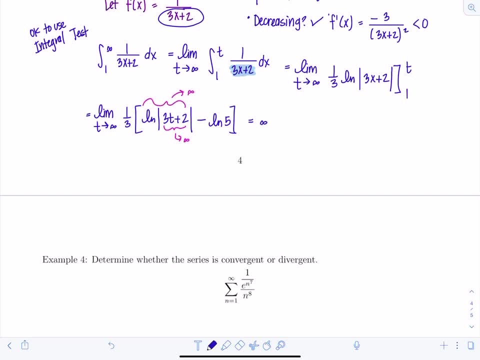 Well, this means that the sum n equals 1 to infinity, of 1 over 3m, 3n plus 2 also diverges by the integral test. Okay, And maybe you had an idea that that was going to happen, because this reminds you of the harmonic series 1 over n. 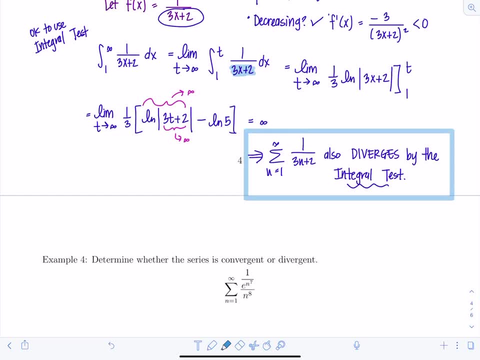 It's just now. it's 3n plus 2. So it's pretty much shrinking or growing, however you want to think about it At the same rate as the harmonic series right Now, if you had something with an n squared in the denominator. 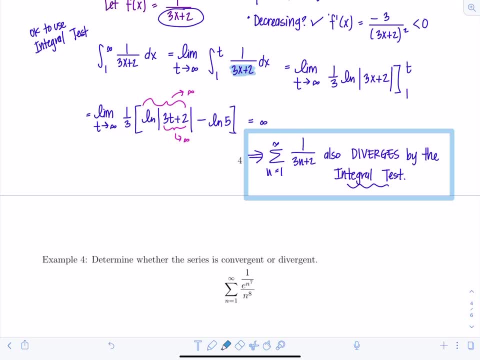 then that would grow like a p-series with p equals 2. That would be shrinking faster, So you would expect something like that to converge. So just keep that in mind, All right. One more example here: Determine whether the series is convergent or divergent. 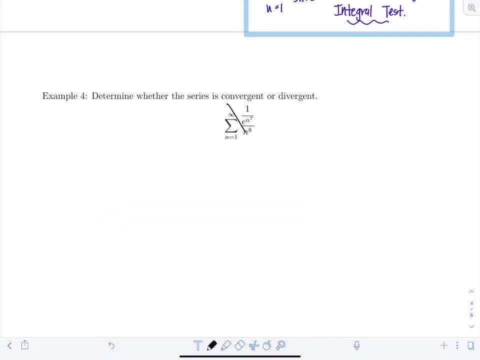 And you know what. This is not written correctly. Hopefully your version This is a little different. This should be: the sum n equals 1 to infinity. The e is raised to the 1 over n to the 7th And then in the denominator we have n to the 8th. 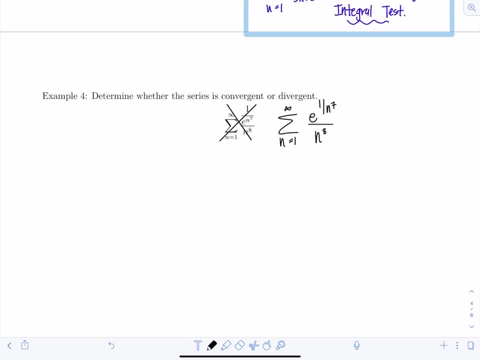 Okay, I'm just going to go straight to the integral test. We're going to consider the function f of x, which is equal to e. Now, this is e to the 1 over x to the 7th over x to the 8th. 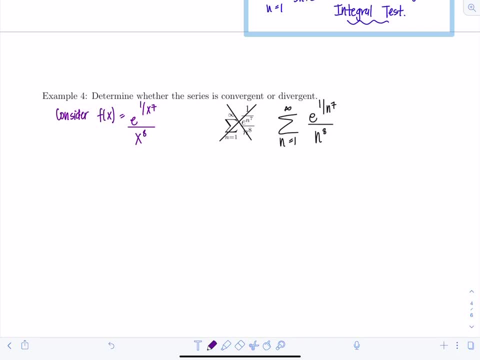 Okay, Good, Now is it continuous on the interval from 1 to infinity. Well, what's the domain for this function? Well, the only value for x that I'm not allowed to use would be 0, right, All x's. 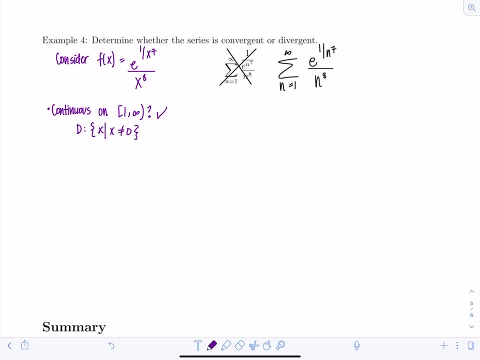 So we're good on 1 to infinity. no problems there. Is it positive? Well, I know, e to the x is always positive, x to the 8th is always positive, so we're fine. What about if it's decreasing? 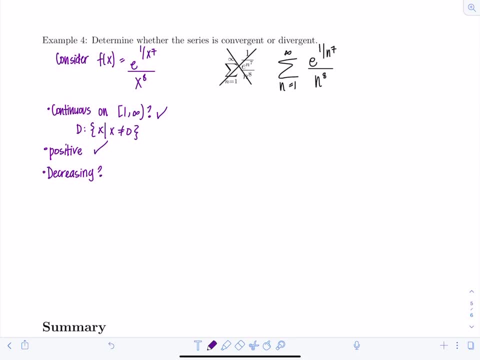 Well, I need to look at its derivative now. Okay, let's rewrite it. so we're ready to take the derivative. This is e raised to the x to the negative, 7th over x to the 8th right. Okay, 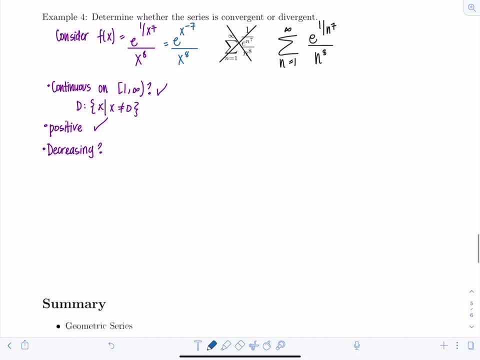 So I'm going to have to use the quotient rule. So f prime of x is going to equal. I have the denominator x to the eighth times, the derivative of the numerator, So derivative of e to the x to the negative seventh, is going to be e to the x to the negative seventh. 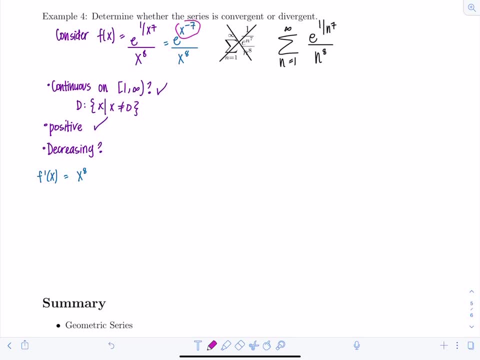 And then by the chain rule I have to multiply by the derivative of the exponent. So I'm actually going to have a negative seven, x to the negative eighth right And then e to the one over, x to the seventh. So that's low to high, if you think of it that way, minus the numerator, So that's e to the one over x to the seventh times derivative of the denominator, which is eight, x to the seventh, over denominator squared. 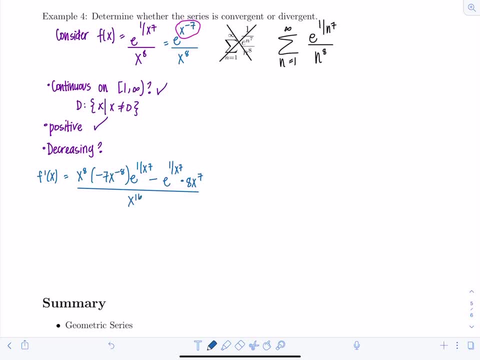 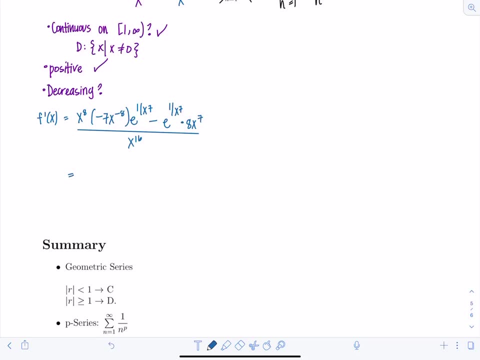 x to the 16th. And remember, I just want to investigate whether the derivative is positive or negative. So let's see. Can I factor out a common factor? Yes, I can take out. watch this. I can factor out the e to the one over x to the seventh right. 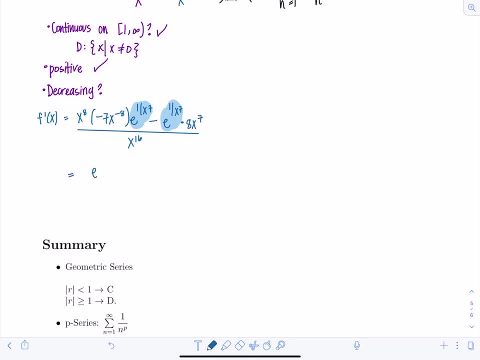 Okay, so I take that out. e to the one over x to the seventh. What am I left with here? Well, I have this: x to the eighth is going to cancel with x to the negative eighth. So all I have is negative seven minus eight. x to the seventh. 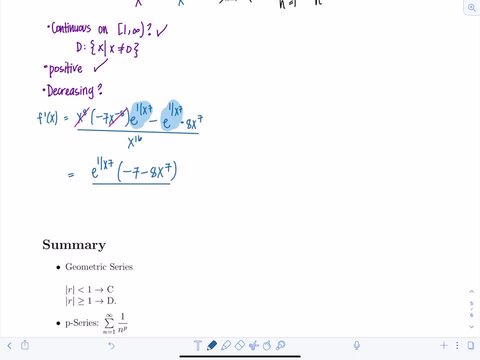 Oh, that cleaned up nicely. over x to the 16th. Okay now let's look at this: e to the one over x to the seventh. that's always positive, right? Think of your graph of e to the x. x to the 16th. 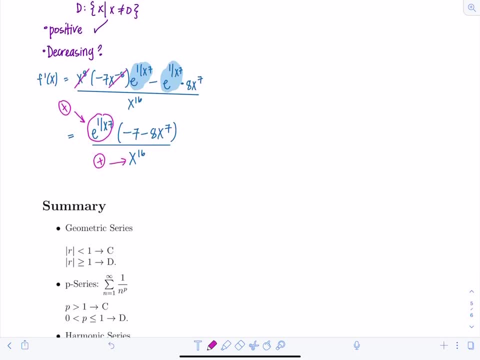 x to the 16th. that's always positive also. Now what about negative seven minus eight? x to the seventh? Remember we're only considering x's from one to infinity. x is always greater than or equal to one. So if I'm only plugging in values for x that are greater than or equal to one, negative seven minus eight times something greater than or equal to one, this is always going to be negative. 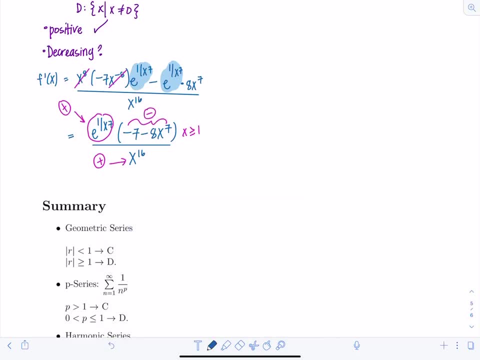 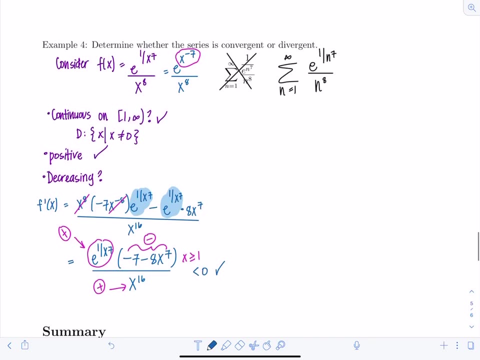 So for sure I can say the derivative is negative on this interval, So it's decreasing Great. All that means is I'm allowed to use the integral test now. So let's do it. So we have the integral from one to infinity of one over. 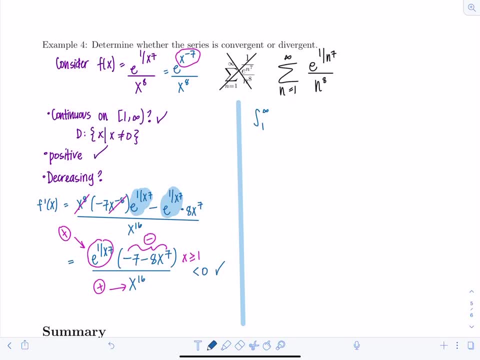 or let me rewrite it as e to the x to the negative seven. So we have the integral from one to infinity, of x to the eighth, over x to the eighth dx. good, so this is an improper integral. I'm going to rewrite this now as the limit, as t approaches infinity of the integral from one to t and then the denominator. I'm going to write it as x to the negative eighth and then e to the x to the negative seventh dx. 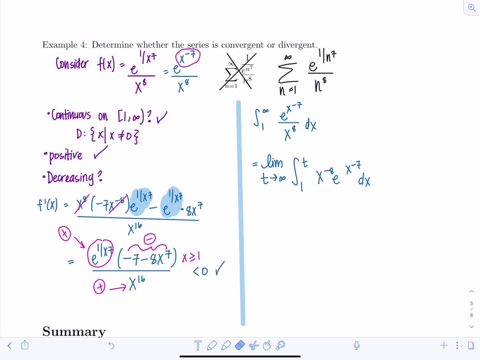 No negative there, All right, All right. And here, hopefully, you can see that we're going to need to do a u substitution. We're going to let u equal x to the negative seventh, the exponent here, and then du would be negative seven. x to the negative eighth, dx, which we have right here. 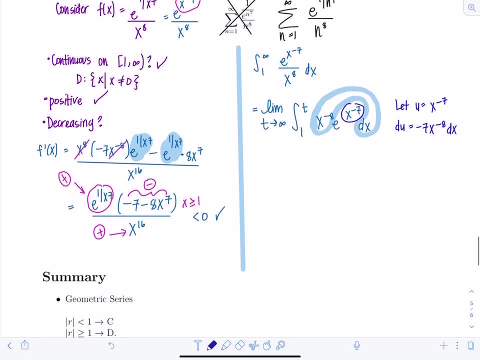 Okay, so I can rewrite this now as the limit as t. t approaches infinity. Now it's up to you. If you're going to leave your limits in terms of x, 1 to t, then you need to indicate that you're not changing them when you do the u sub. So this is: 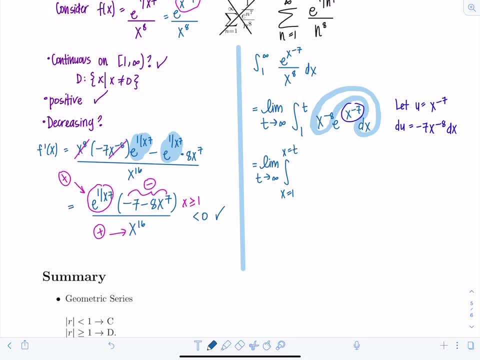 x equals 1 to x equals t. Otherwise change them. okay, And then we're going to have a negative one-seventh e to the? u du. If I anti-differentiate, that's just going to give me e to the? u. 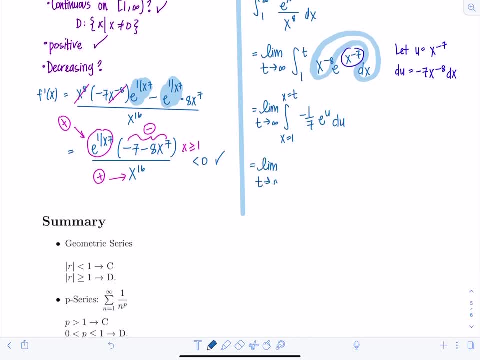 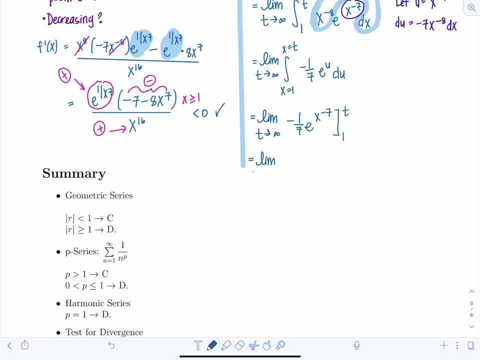 So this is the limit as t approaches infinity: negative one-seventh. e to the x to the negative seventh, from 1 to t. All right now, substituting in our limits of integration, we have the limit, as t approaches infinity, of negative one-seventh. Leave that outside so you don't get all confused. 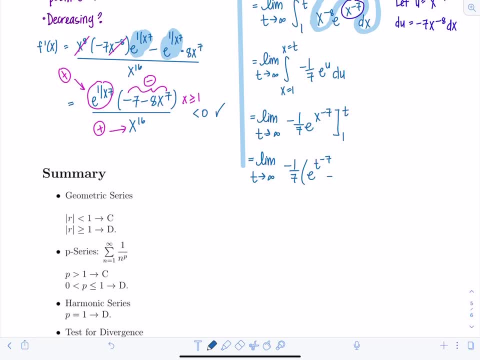 So this is going to be e to the t to the negative seventh minus e to the first, So t to the negative seventh. As t approaches infinity, that's 1 over t to the seventh. So this exponent is going to be approaching zero And e to the zero is going to be 1.. So this limit here is negative one-seventh. 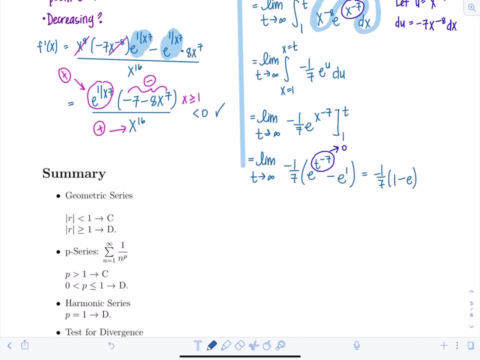 times 1 minus e, which I can rewrite as one-seventh times e minus 1.. I don't really care what it comes out to. All I care is that it's finite and the improper integral converges, So what this means is my. 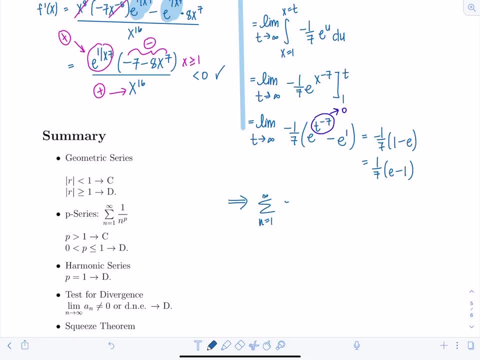 original series. n equals 1 to infinity, of e to the 1, over n to the seventh, over n to the eighth. also converges by the integral test. Okay, nice job. Now to summarize what we've covered thus far in the chapter. 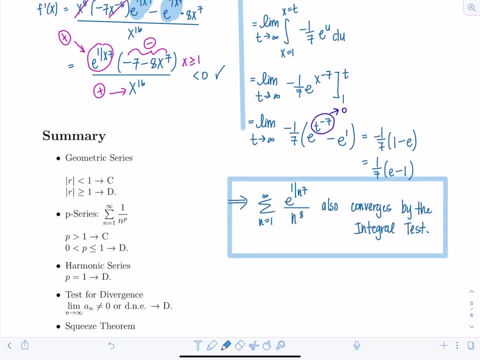 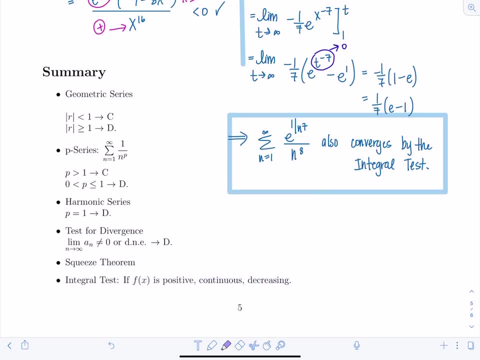 take a look over here on the left And we've gone over. remember, if the common ratio is less than 1, the series converges. If the common ratio is greater than or equal to 1, it diverges. P-series: we've looked at p-series today. If p is greater than 1,.